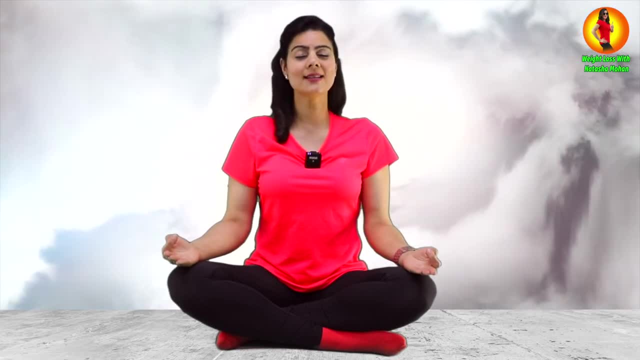 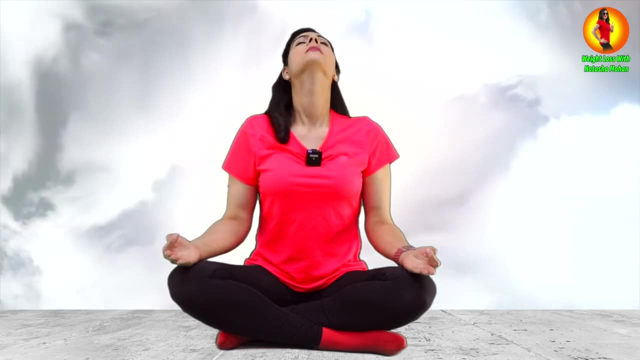 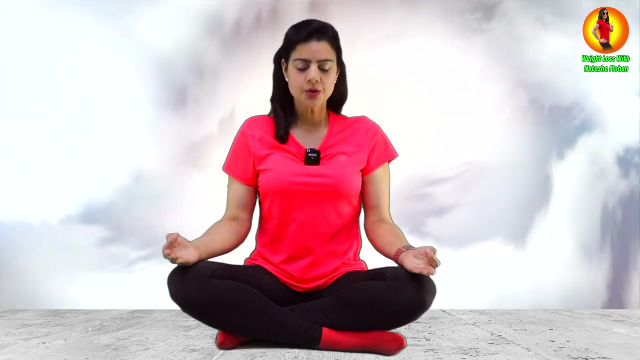 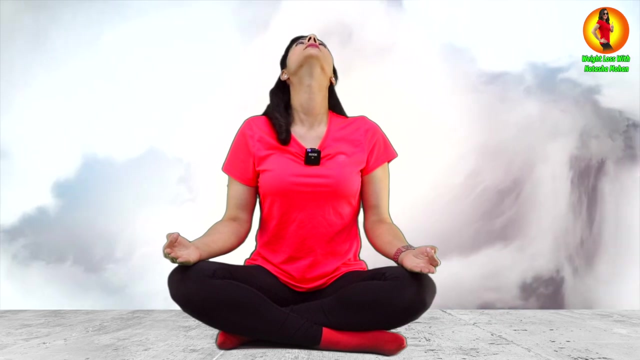 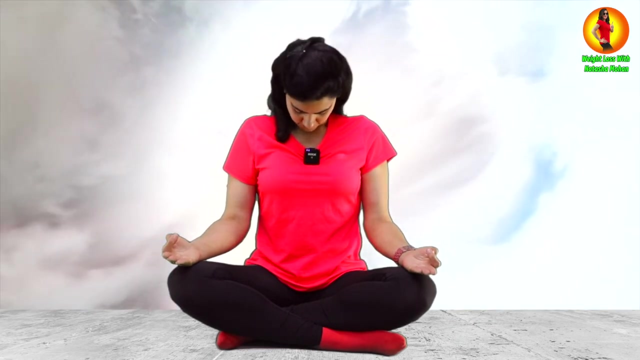 exercises. To begin with, we are going to exercise our neck: Exhale and go down, Inhale while you go up. It's your choice if you want to keep your eyes closed or if you want to gaze at the ceiling. 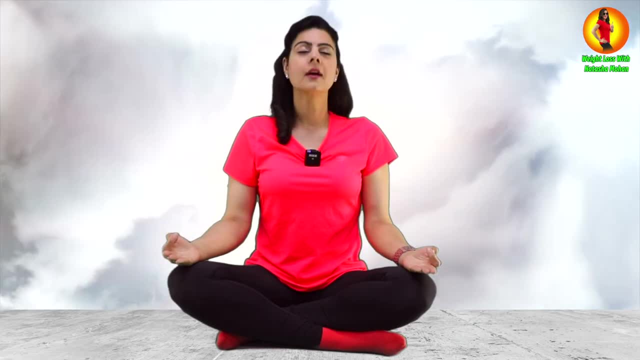 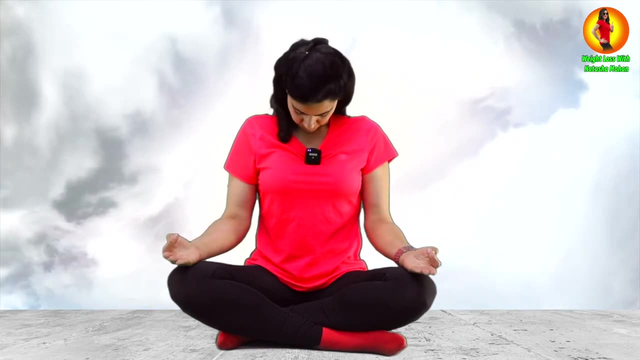 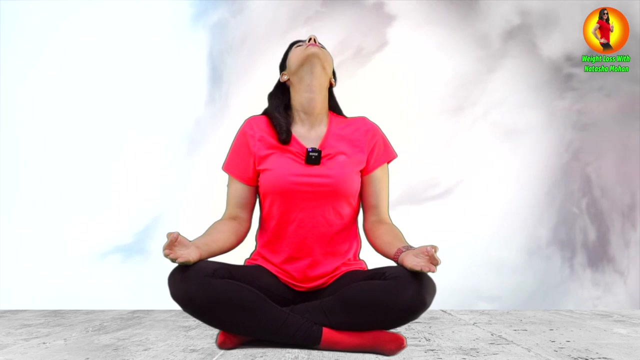 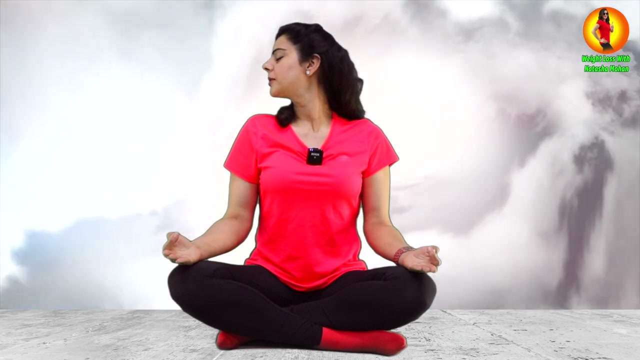 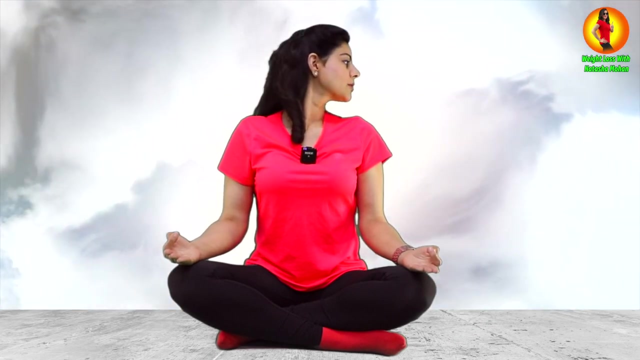 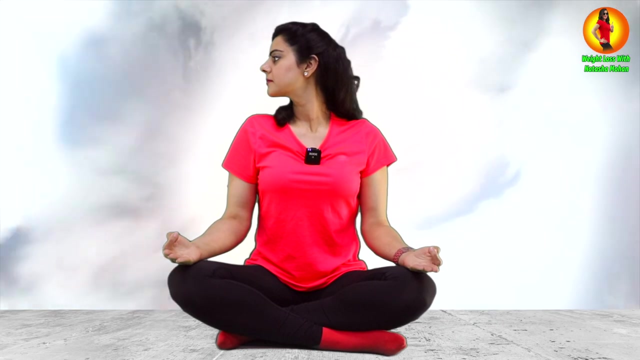 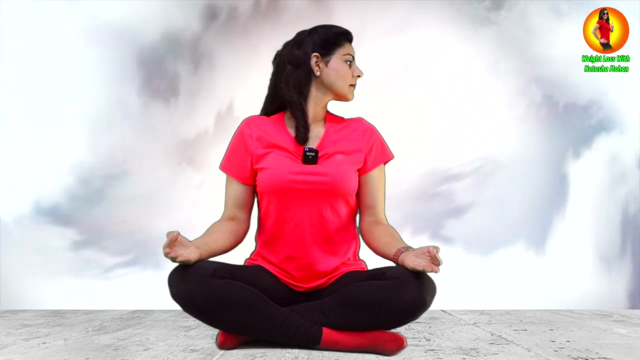 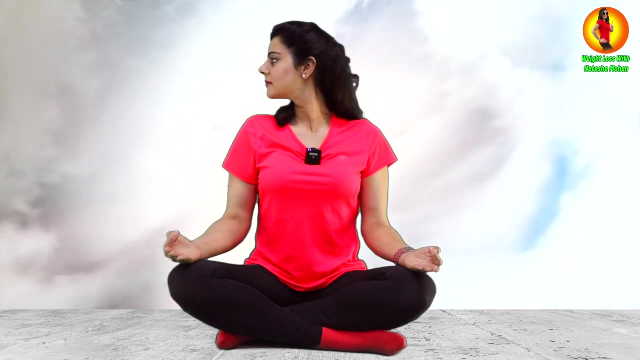 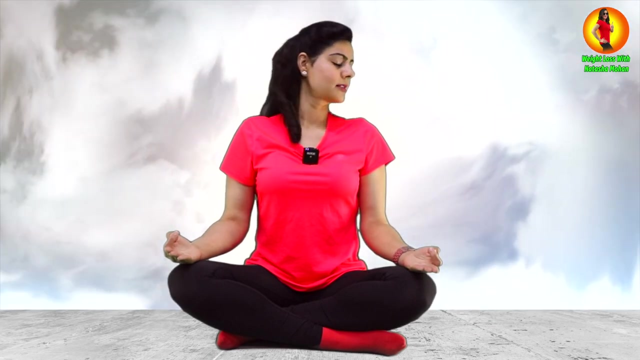 Keep your neck moving, Slow and steady. Feel this stretch, Feel all your neck muscles relaxing. Now, moving sideways, Your chin will be parallel to your shoulder, Left to right And right to left, Keeping your spine straight at all times. Now it's time to exercise the shoulders. We are going to keep our hands like this and 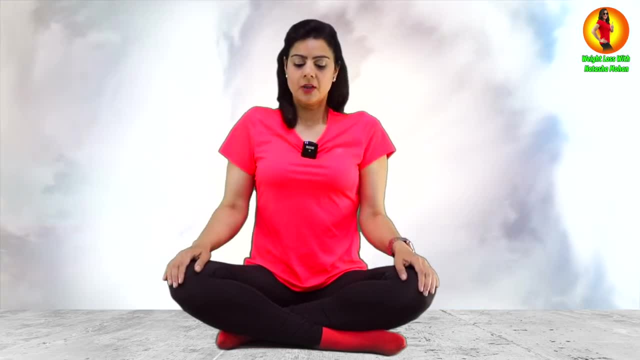 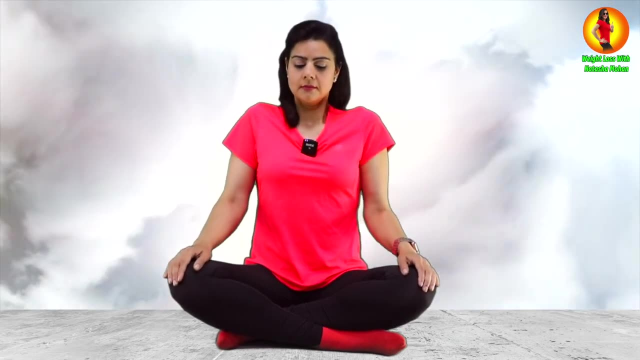 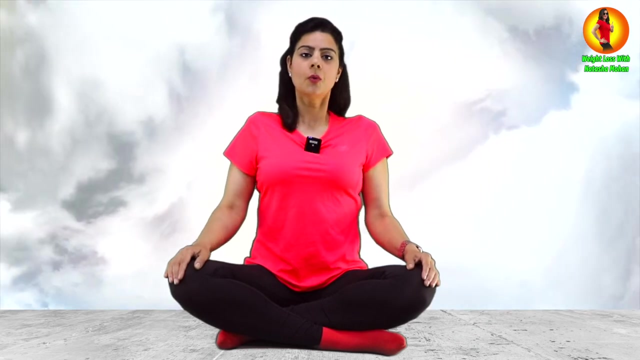 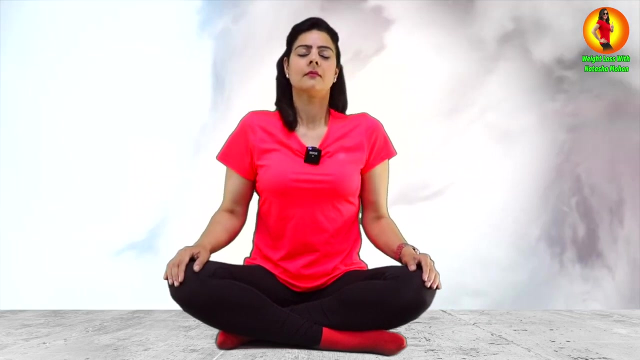 make circles with our shoulders, Moving only our shoulders and keeping the whole body still. Make as big circles as you can, Keeping your movement slow and steady. Now, this is called the Metta steady. Often we overlook the upper part of our body and forget to exercise and 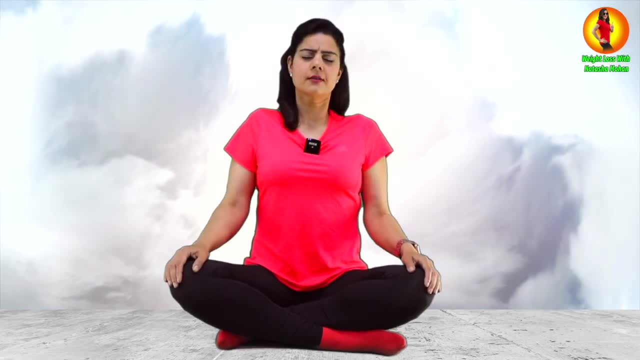 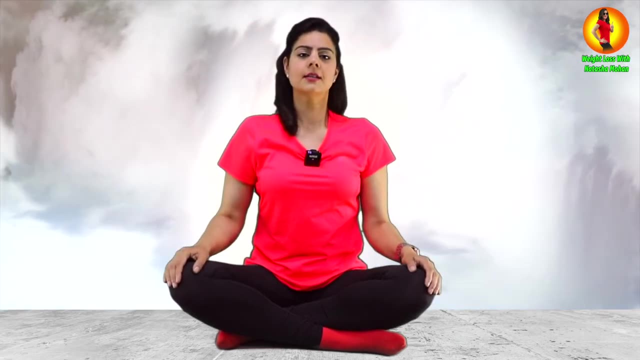 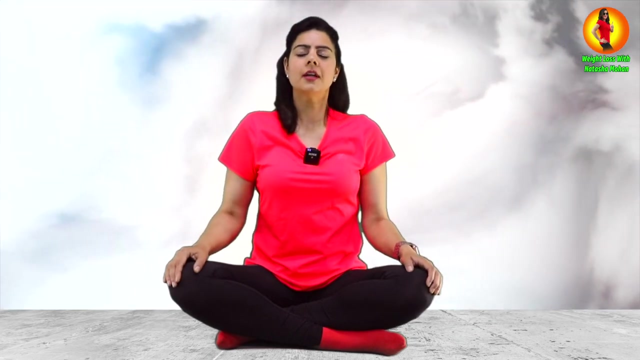 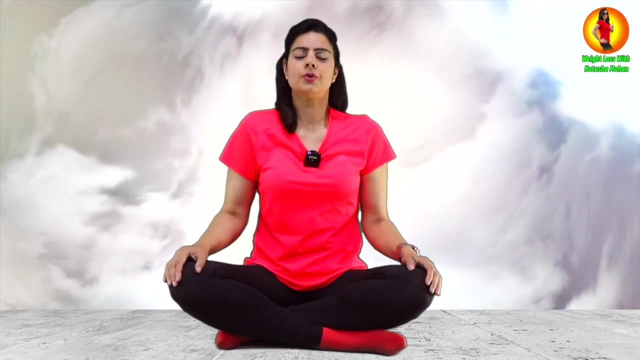 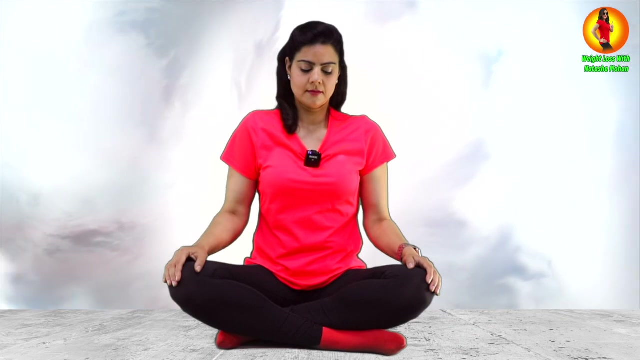 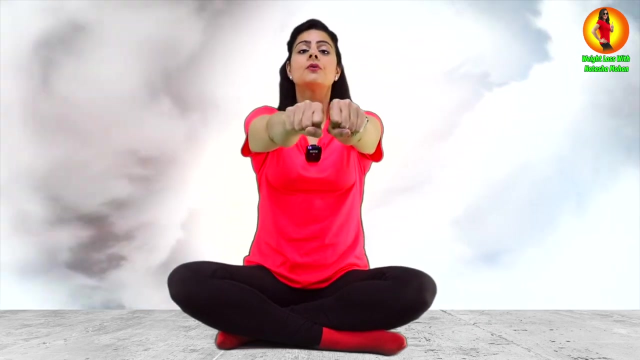 that's when we feel and feel so stressed at the end of the day. Now let's rotate it anti-clockwise, very slow movements, feeling every inch of your shoulders, moving in round circular motion. Now it's time to exercise the wrists. You're going to close your fists. 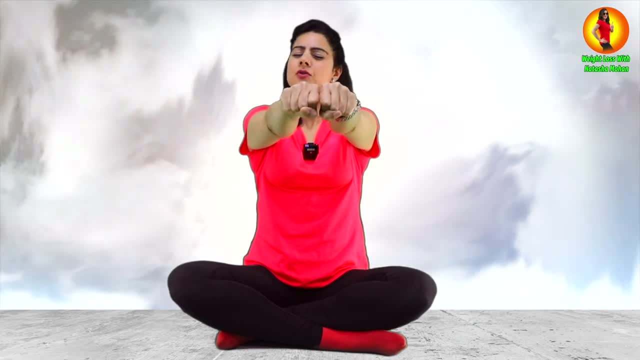 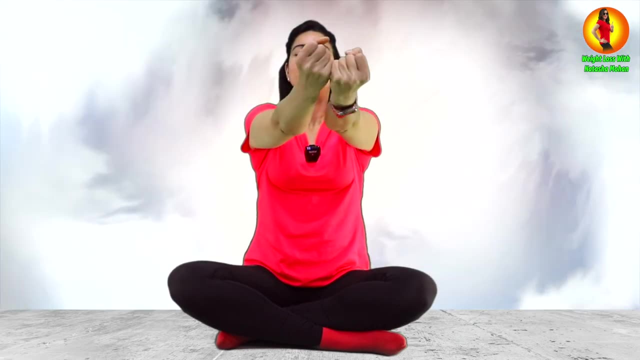 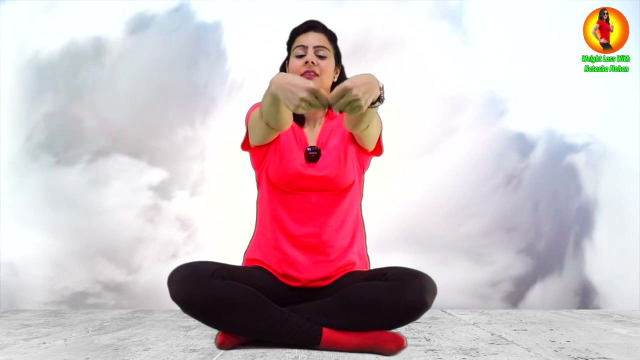 like this: keep your arms straight, stretched, no bending elbows, and you're going to rotate your wrist while keeping them touched to each other. Make sure you're not doing this. they should be touching each other while you rotate them. That's when you're actually going to feel the stretch and the 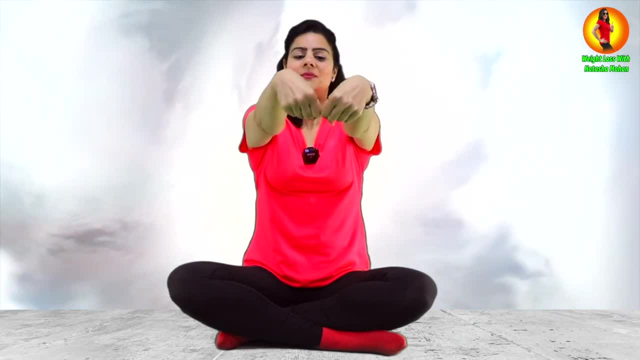 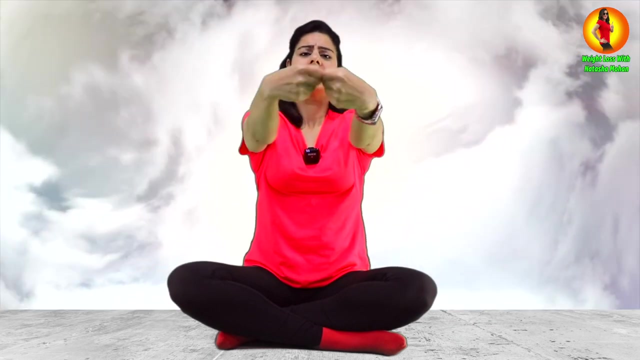 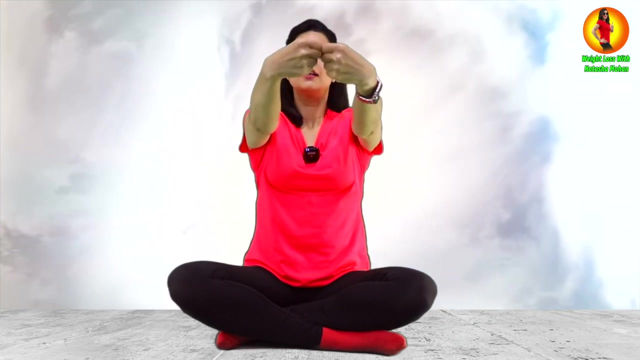 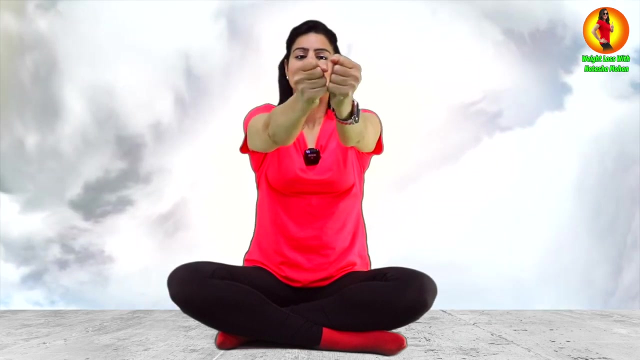 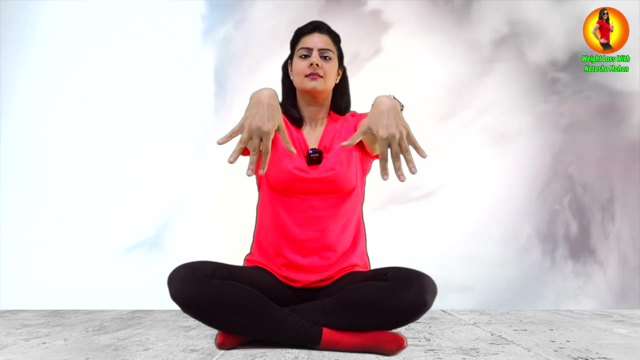 relaxation, Now anti-clockwise. These simple exercises, when performed early in the morning, can actually help you get rid of all the negativity and open your mind to all the positive thoughts Which are going to help you sail through the day. Now time to move on. We're going to do our wrist exercises. Just lift it up and drop. 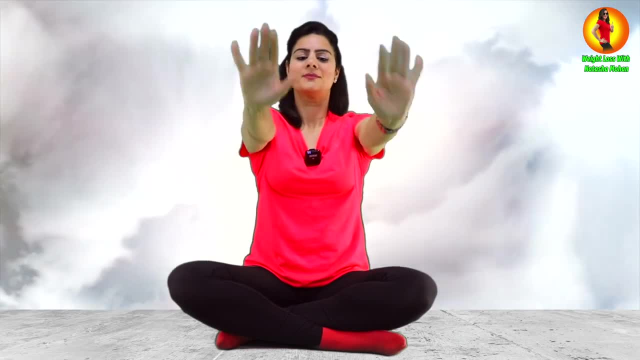 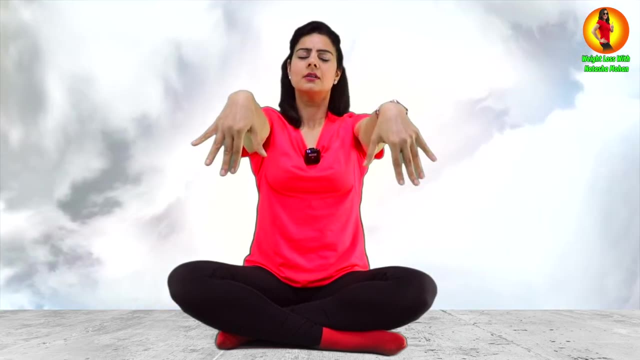 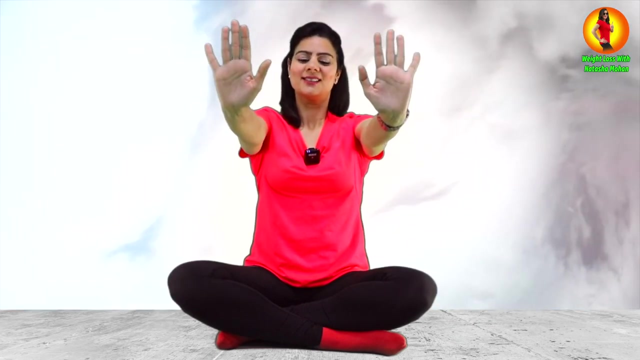 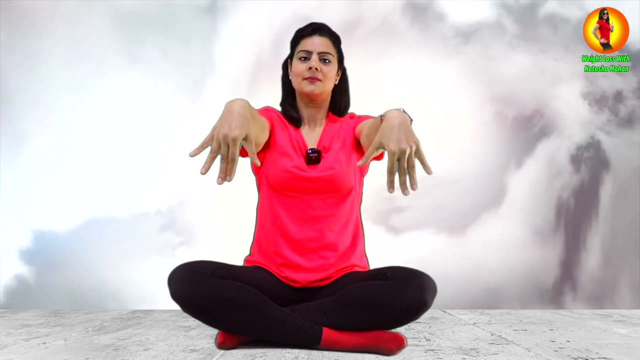 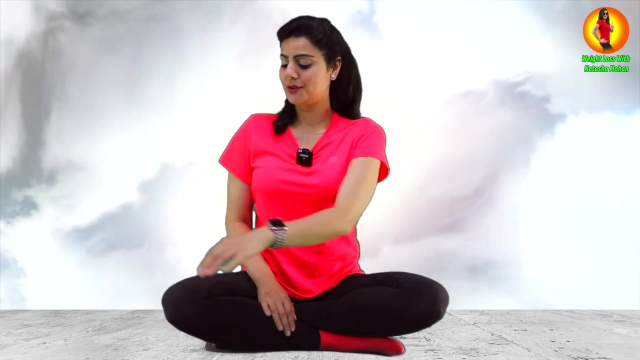 Lift it up and drop A slight jerk and you're going to feel the tension in your shoulders. You will get a little relaxed. Sindhuya爷, I'm just notrek this Rural exercise. The next beginner-friendly yoga exercise is for your torso and your spine. 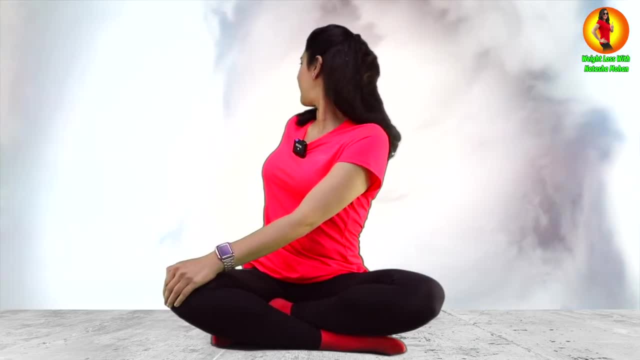 The next beginner-friendly yoga exercise is for your torso and your spine. Keep one arm like this, Then the other behind you and turn all the way back. Keep one arm like this, Then the other behind you and turn all the way back. Ho niveata. 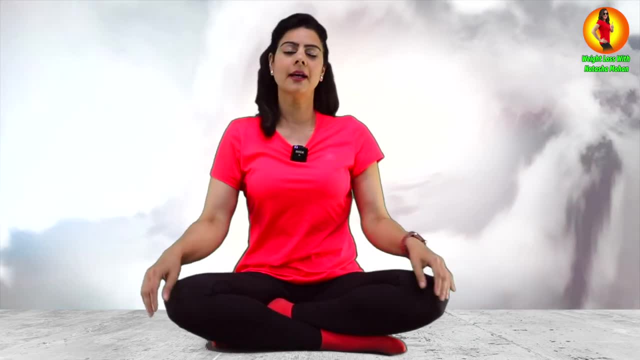 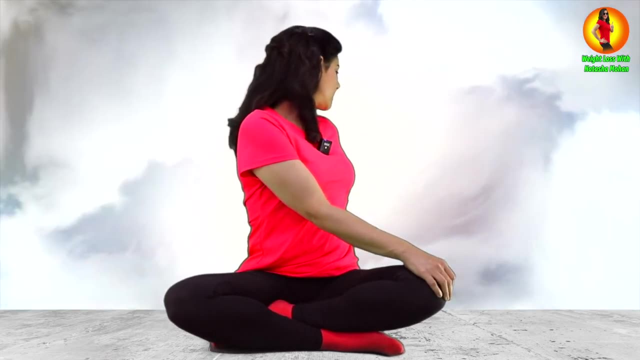 Hold it till five counts. come back again, then again with the other hand, again hold it till five counts. it's going to help you relax your back muscles. keep your spine straight. you can feel the stretch. it's very rejuvenating. 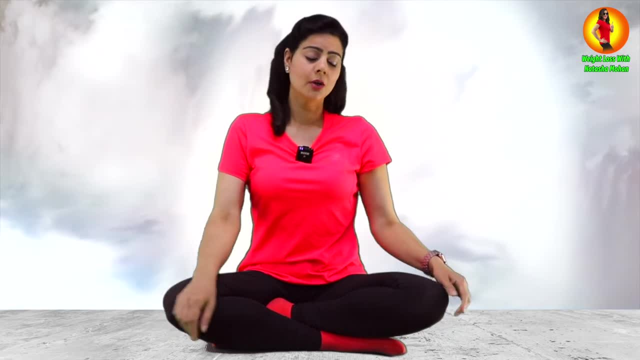 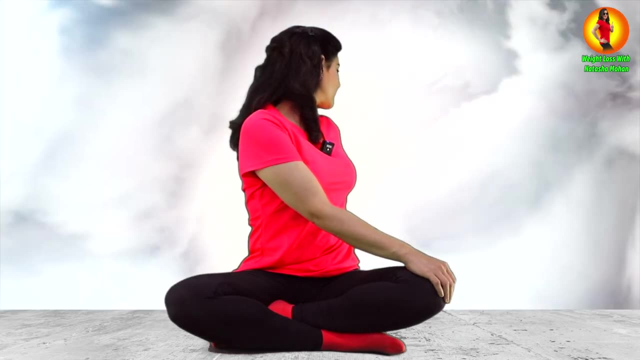 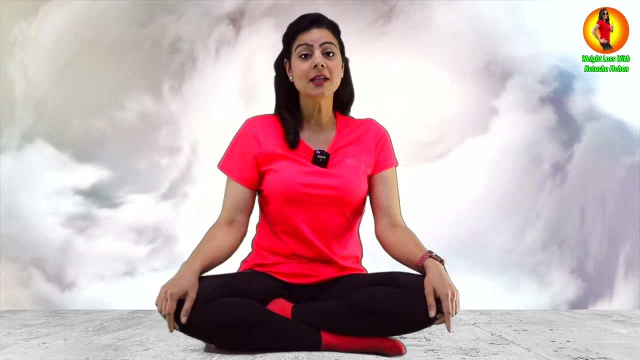 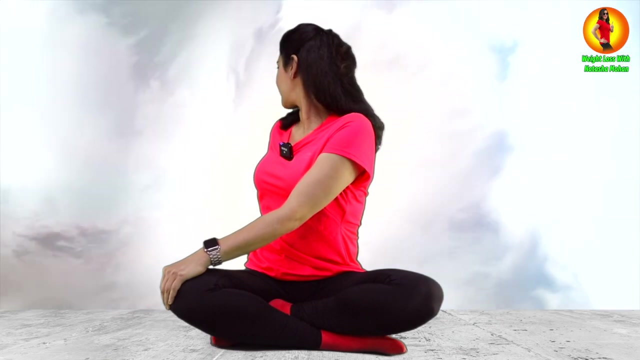 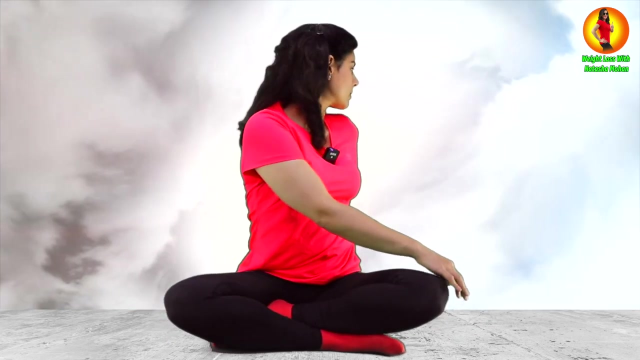 You are going to feel a world of change when you keep practicing these exercises on a daily basis. Consider this as me time and get to know yourself better. Try and understand what led you to gain so much weight. What was the main cause which stopped you from losing all the excess weight? 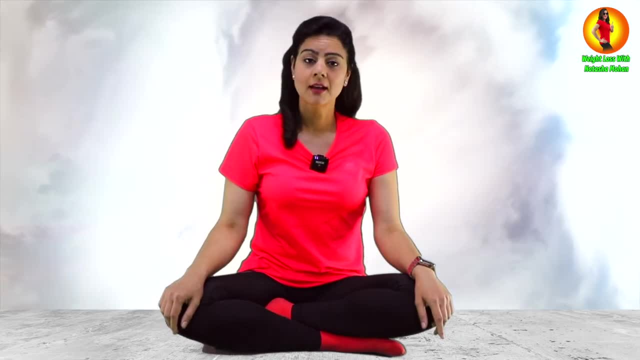 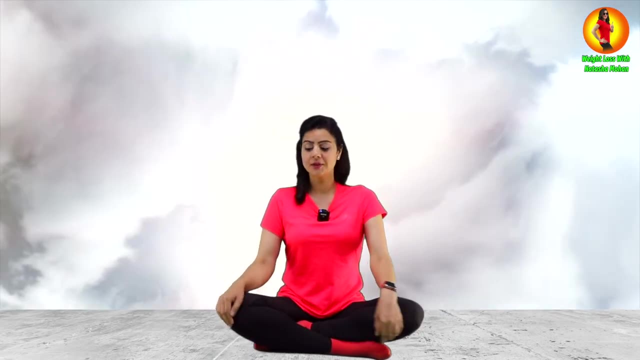 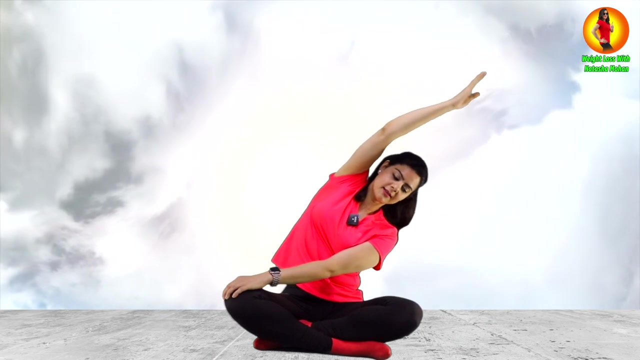 This way, you will be able to build up your inner strength and get over any hurdle, come what may, in your life. The next yoga exercise we're going to put one arm like this, like we did in the previous exercise, Take the other one right up there and bend sideways. 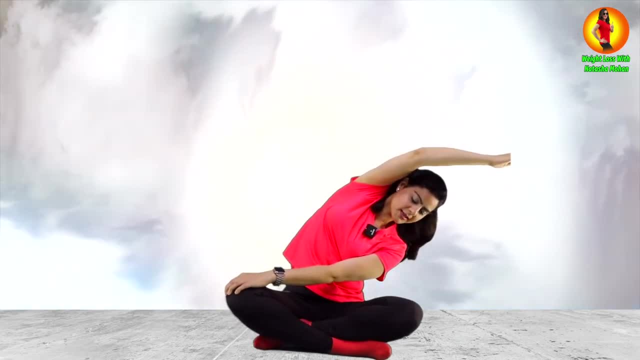 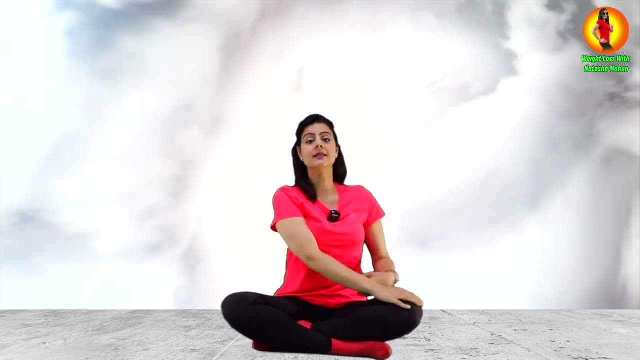 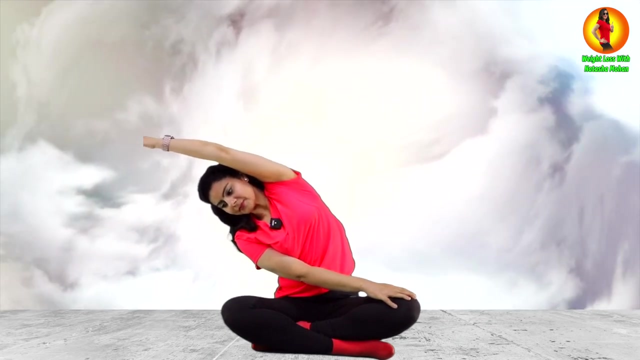 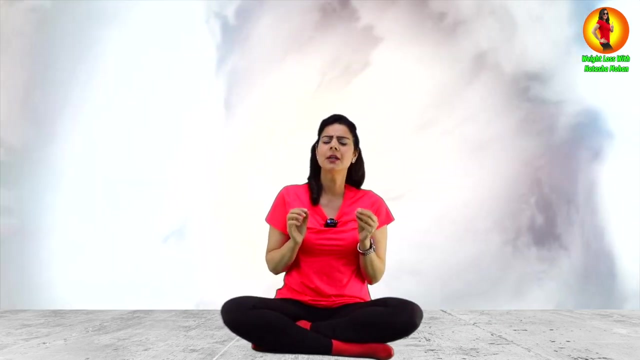 We'll try and exhale when we go down. when we come up, inhale with the other hand and exhale When you're exhaling. make sure to hold in that position for minimum three to five counts, and that is what is going to benefit you immensely. 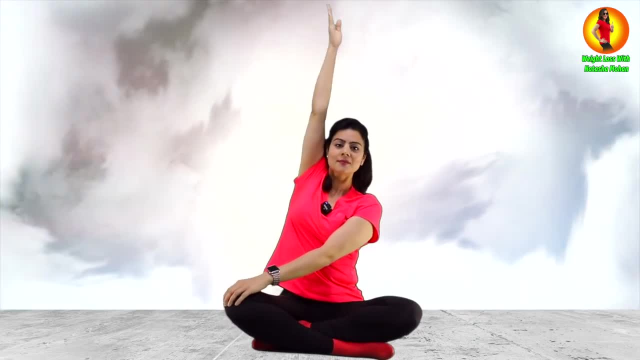 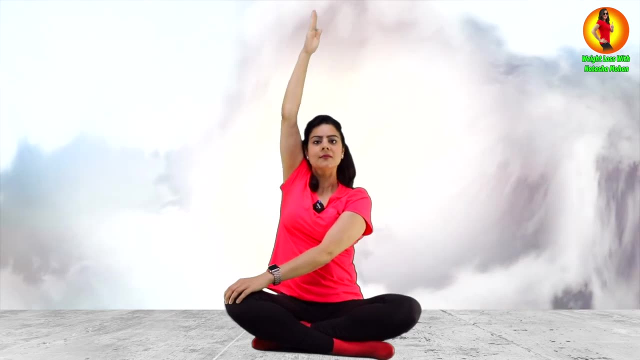 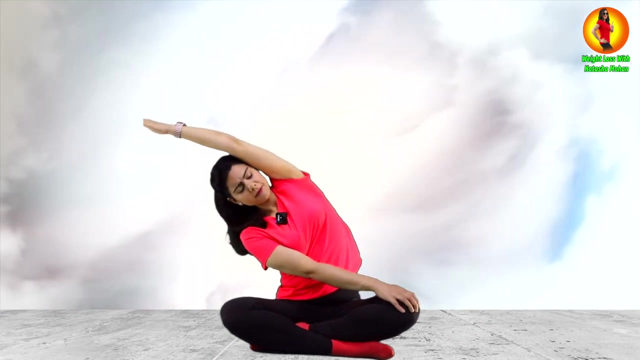 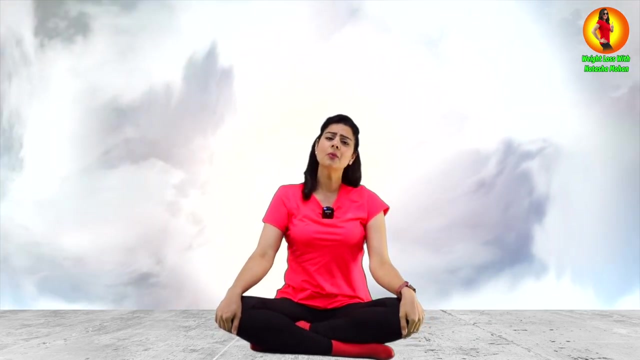 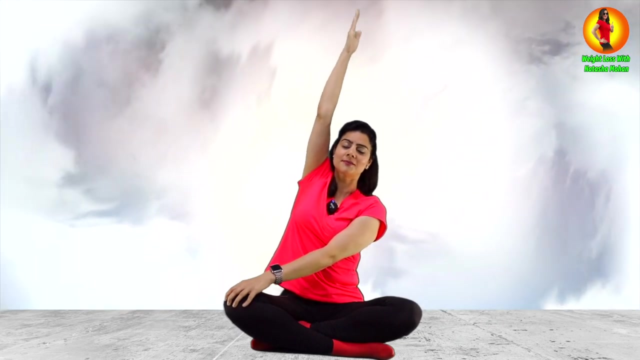 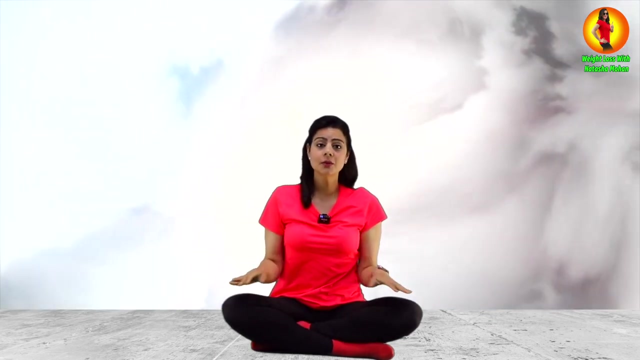 Just like this, You're actually going to learn to use your body efficiently, to continue with your daily chores and make the most of it. That's exactly what the purpose of the human body is and what it should be. You will get to regulate your blood circulation. 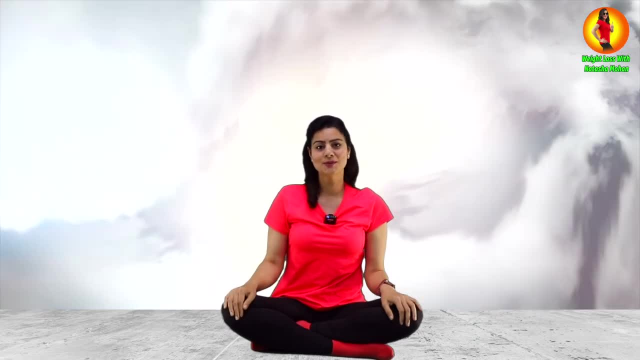 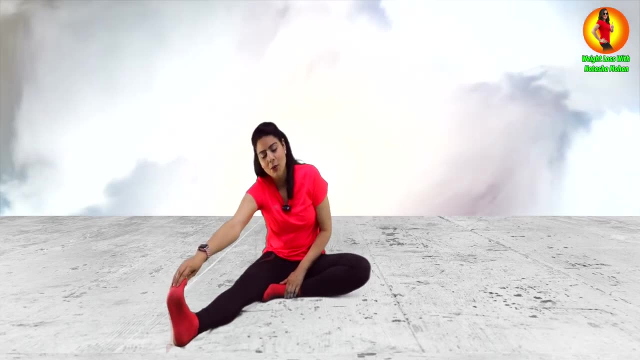 and your body will be thankful to you for doing these exercises. For the next exercise, we're going to sit with our legs folded- one leg folded, the other one straight. If you're not able to hold up to your toe, then you can hold right here.